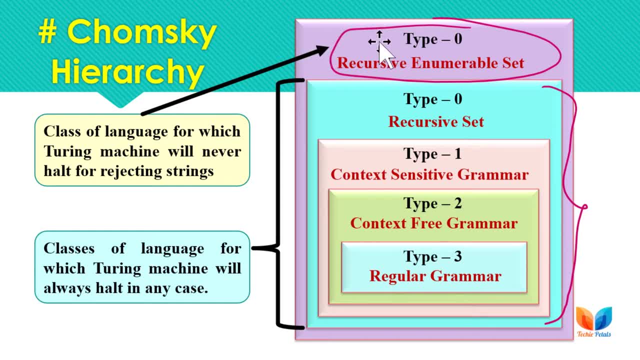 rejection case. So let's start with this. problem means whether the machine, whether the machine by machine. we mean that a program or a Turing machine For a given input string will eventually halt or not. we are comparing it with the simple program of any language. if we are having an infinite loop in the program and we are giving 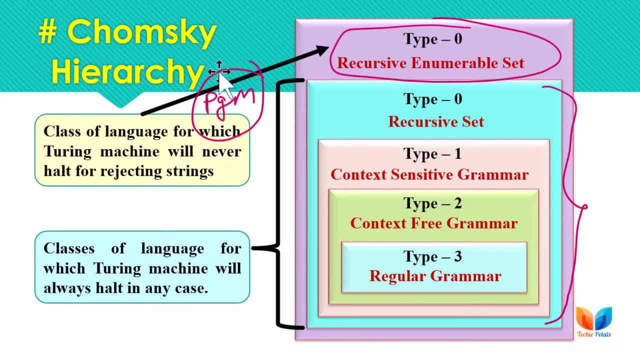 some input that is not according to the program. So let's compare these things with the simple program that we have run so many time. So if the string provided to the program is in the language so the machine will end means it will give the result in the program. So 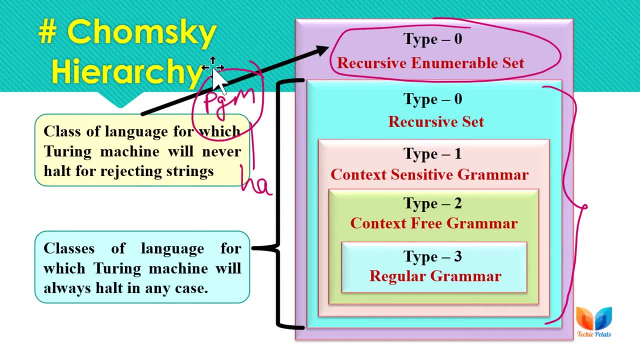 required output. but if that machine, if that string is not in the language or not according to the program statement, program logic, then the machine may loop forever, okay and may, goes to the infinite loop and will will never halt. to even halt, reject, state mean it cannot give the result. so that case means we cannot. 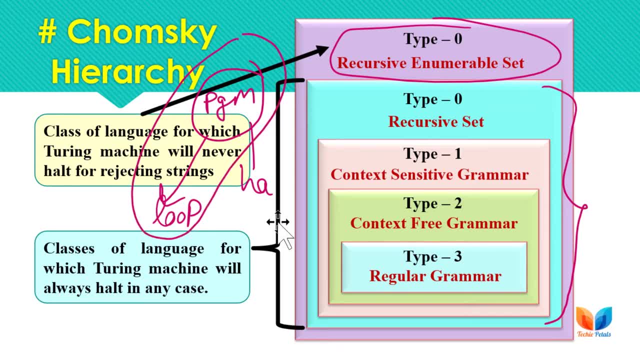 predict this case. we cannot predict this case, but we can predict this case. that program will give output for all the string that are in the language. so the prediction is very much possible for this recursive set, but not possible for recursively enumerable set means whether the program will give output or 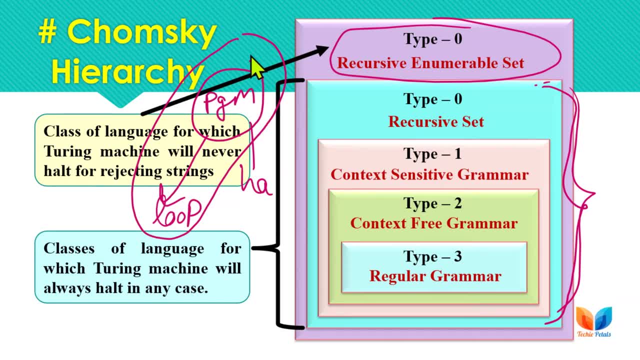 halt or not, or it will go to the infinite loop. so this problem comes under the undecidable problem category, means the problem that needs to be solved cannot have a particular solution. we cannot predict whether this program will eventually halt or not, so such problem is undecidable. so before discussing this problem of 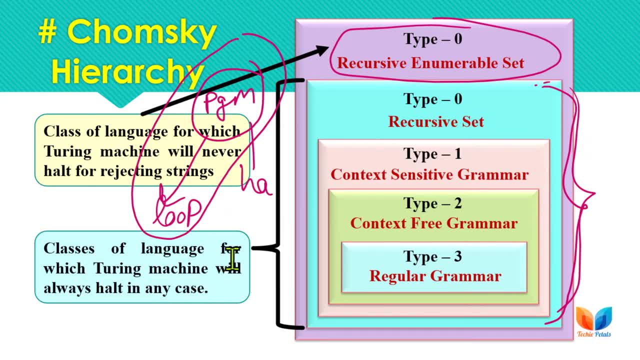 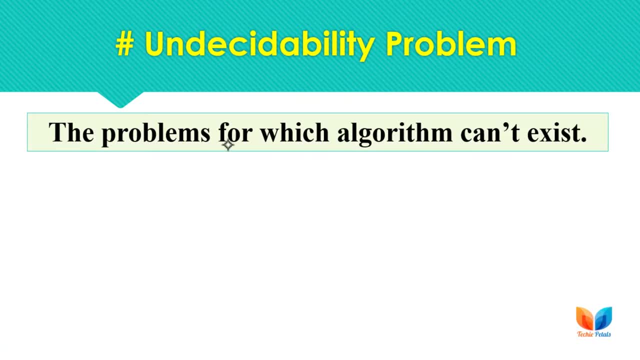 turing machine. let's discuss about the undecidability as this. so undecidability problem is a problem, or are the problems for which algorithm cannot exist means we cannot have the solution corresponding to this, corresponding to all the undecidable problems? okay, so, for example, the fermat's last theorem. 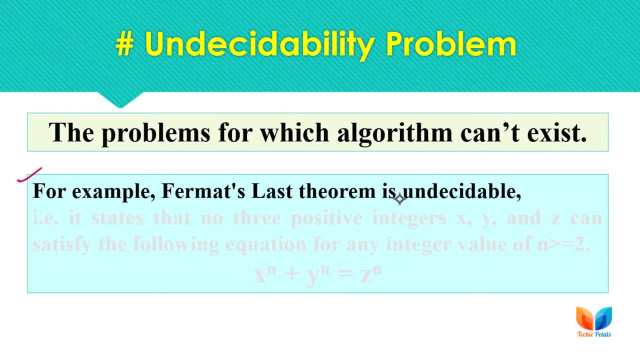 is undecidable, and it is already proved to be undecidable because we cannot find we cannot find the three positive integers x, y and z for this particular equation, for the value of n greater than equal to 2 means we cannot find the solution of this equation. 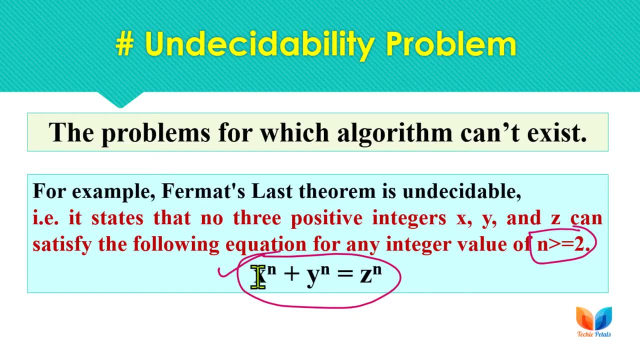 by x, by a appropriate values of x, y and z as positive integers for all n greater than equal to 2. so this problem is already proved to be undecidable. because we cannot have the algorithm that can solve this problem, we always stuck into the loop: or we cannot have a. 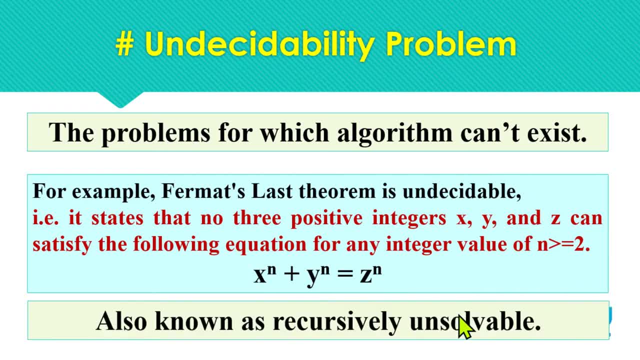 accepting state for this particular problem. so this is also known as means. undecidable problems, also known as recursively unsolvable problem, means we cannot solve them even with the lots of try and recursively analysis or anything. so now the examples of undecidability problem so we can categorize. 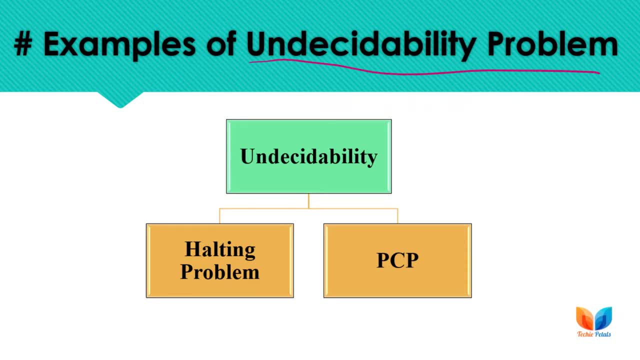 or we have two types of here, two major categories of undecidable problems, examples as halting problem and the pcp problem- halting problem of turing machine- and again we have a string type or a different type of problem, that is, pcp, post correspondence problem. that is also. 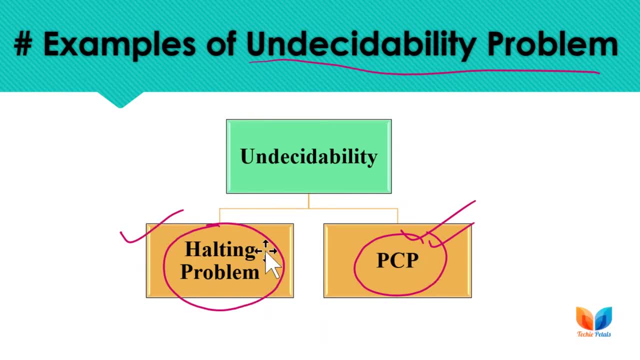 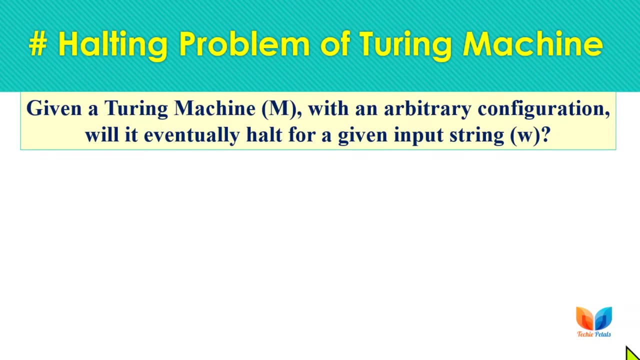 undecidable. but for this lecture we are solving only, or we are proving only, the halting problem. in next lecture we will be continuing with the pcp problem or the post correspondence problem. so let's start with the halting problem. the halting problem is related to the turing. 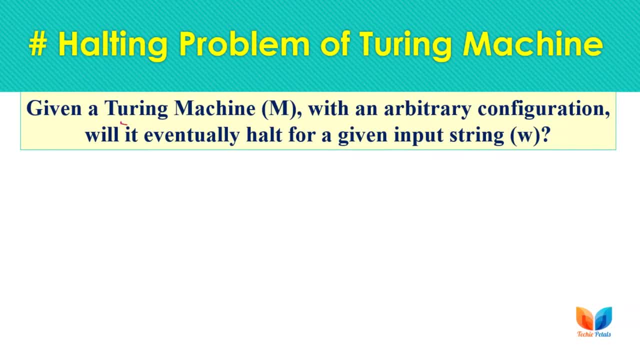 machine. so if we are given with the turing machine m- by turing machine we mean that we are given with a program N with some specific configuration means for a particular problem- if we are having a program M or a Turing machine M, will it eventually halt for the given input string? 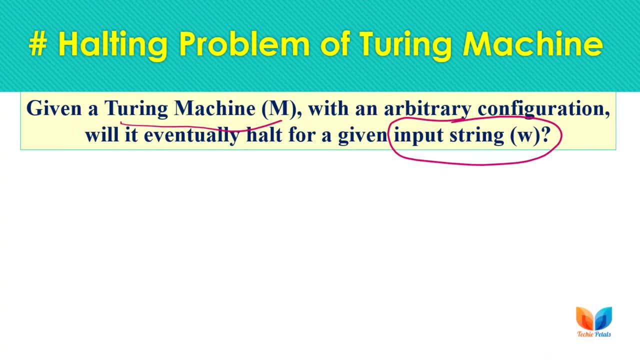 So we have to solve this question means: can we answer this question? will the program M or the machine M will eventually halt for this string W or not? so this is the problem: Can we predict this? that it will give a result means it will halt for this particular string. 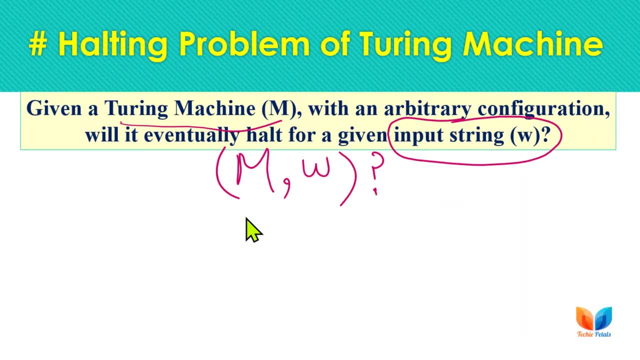 or not, So by halting problem. so this is the halting problem of Turing machine, whether this Turing machine will halt or not. but here we have to prove this: that this problem is undecidable because we cannot predict this case means for a machine, we cannot predict for a string. 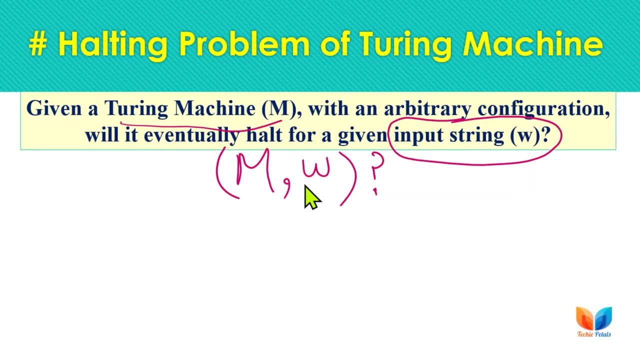 it will halt or not, or it may go into halt, So we are going to infinite loop. we are talking about the string that are not in the language. if the string is in the language, so, as was the case of recursively enumerable set, for all the string, for recursively enumerable set, all the strings belong to the language. 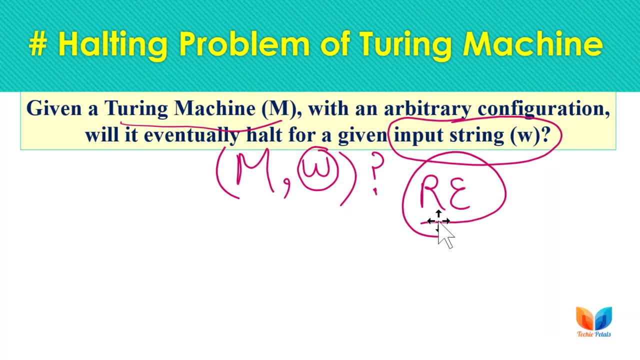 the machine is giving a result means machine will end with the halt except state. But if the string does not belong to the language, then we cannot be sure of the halt means machine will ever halt or not For the rejected string. this is the question. so here, the machine may or may not halt, or? 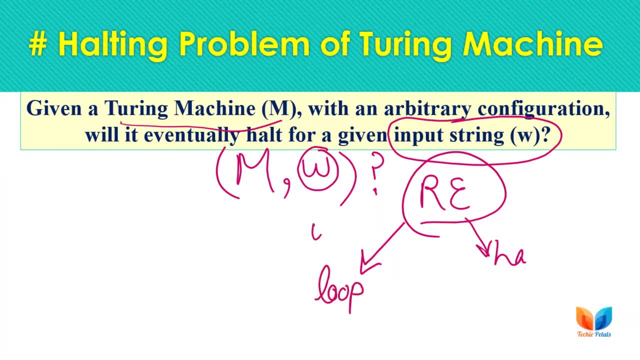 may go to the infinite loop for the string. that does not belong to the language of machine. So this was the case of recursively enumerable set, where all the strings that are acceptable, the machine is giving a result and ending with the halt, except state. 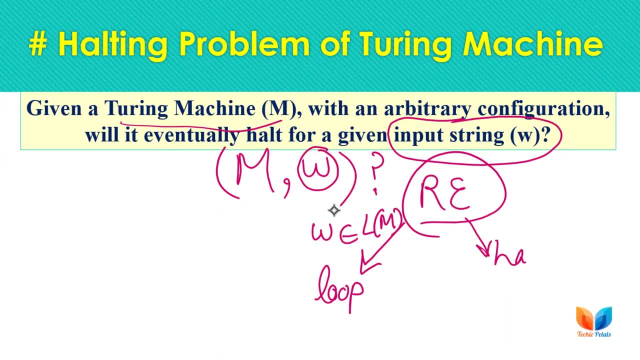 strings or any string will. that doesn't belong to the language of machine. the machine may or may not give the result or may end with an infinite loop, and the machine goes to the may a. the machine will not even end with the halt reject state. so we are not ending with halt reject state here, for the string doesn't. 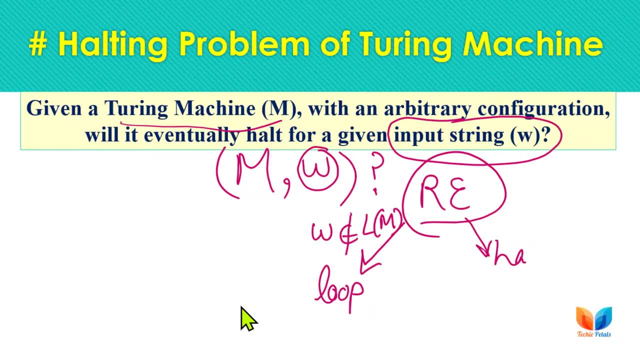 belong to the language, we are going to the infinite loop. so can we predict this case, that machine for that machine, M will go to the infinite loop for this particular string or not. so this is the problem that is halting problem of Turing machine. we cannot predict this case, so we have to prove this, that this 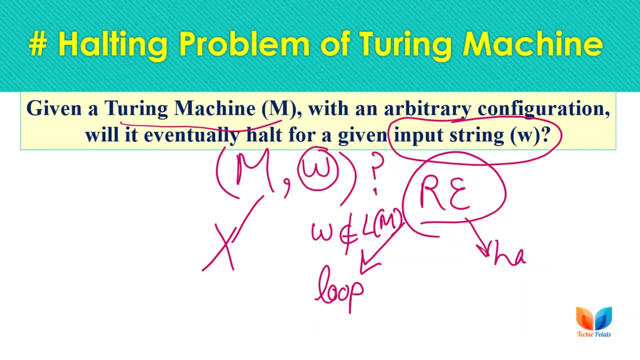 is recursively unsolvable problem. problem: we cannot predict this possibility that whether machine will go to infinite loop or not, before running the string, so before giving the input to the machine. so just problem is undecidable. and we have to solve this problem with the, with a theorem and with the contradiction. so let's start with the lecture here, the, 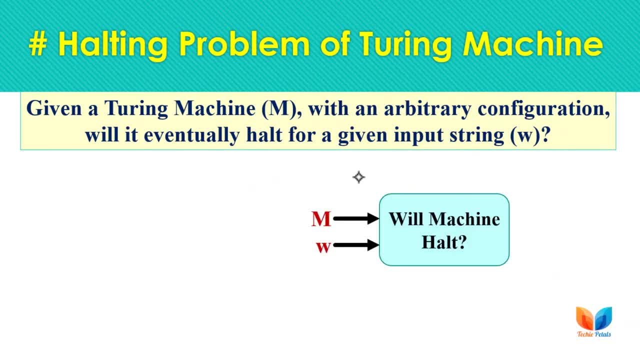 proof of the halting problem. so, reia, proving the solution. we are proving this theorem with the contradiction that we can predict whether this machine M will new forever or will halt, for the W string means that W just saying that doesn't belong to the world machines. R el hela, maki, maki, maki, al lazim yusqu nov ek. 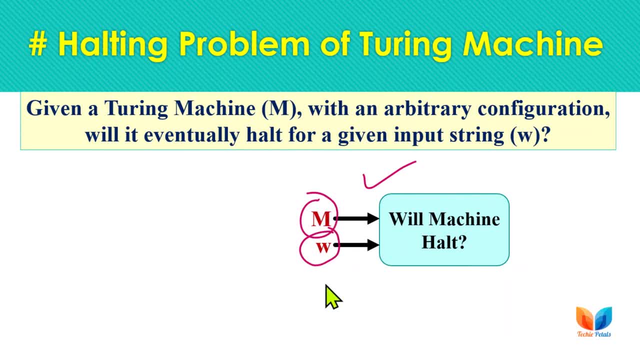 to the language and we have to predict whether the machine will halt or not. so we are assuming- we are proving this with a contradiction- that there is a machine, there is a machine that can take the description of turing machine m and the string w and can predict and can predict the. 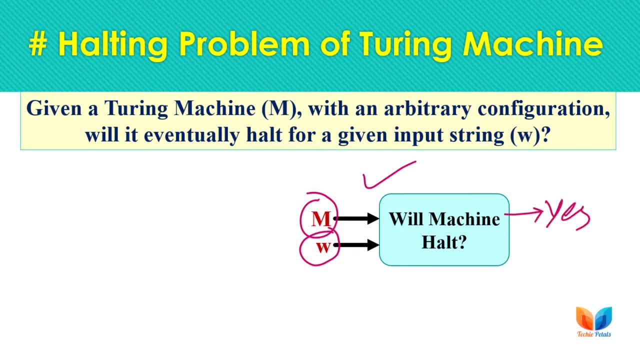 output that, whether the machine will halt, yes or not. okay, for this particular string this machine is, or? by machine we mean that algorithm. this algorithm is giving you a result, whether this machine, for this particular string, will halt or not halt. by not hot, we mean that it may end goes. 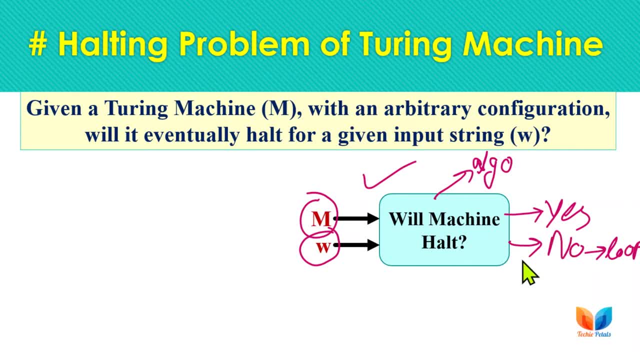 to the infinite loop. so if such machine can exist, then the problem is solvable. but can we have such machine? this is the question. okay, so here can we design a machine which can find out whether a given machine can be halted or not. okay, so here can we design a machine which can find out whether a given machine can exist, then the problem is solvable. but can we have such machine? this is the question. okay, so here can we design a machine which can find out whether a given 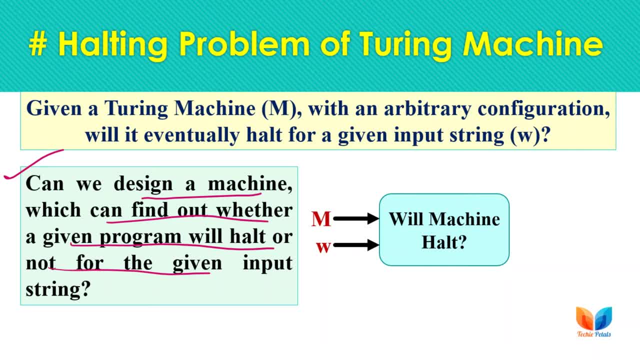 machine can exist, then the problem is solvable. but can we have such machine? this is the question. okay, so here can we design a machine which can find out whether a given program will halt or not for the given input string? so we have to find out this under the halting problem. 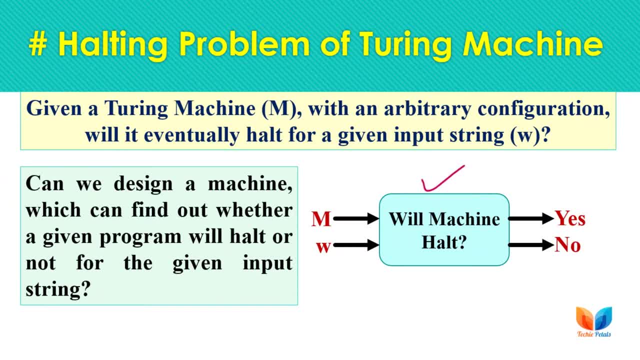 so here this machine, if such machine can exist, it will give a yes if the machine will halt for this string and will give a no if the machine cannot halt for this string w. so don't get confused. it's a simple contradiction case that you have done for the many of the mathematical theorem, so we 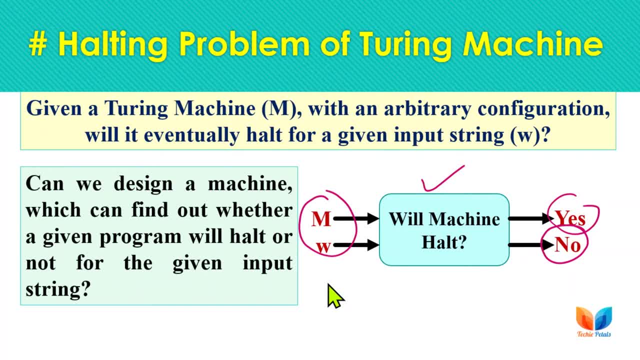 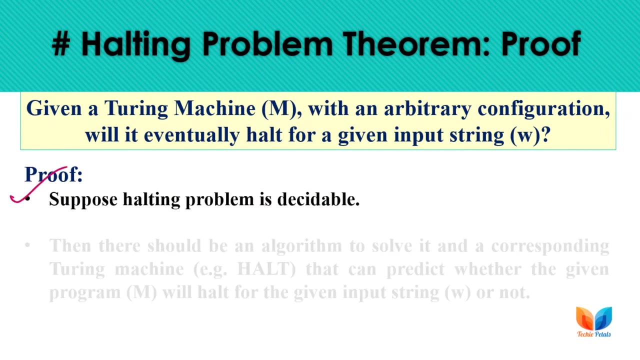 are taking the same case here. so we are assuming that there exist such type of string, such type of algorithm that can predict or that can output whether this machine will halt or not halt for the input string w. so so the proof is by contradiction. so for this we are, we are supposing, or 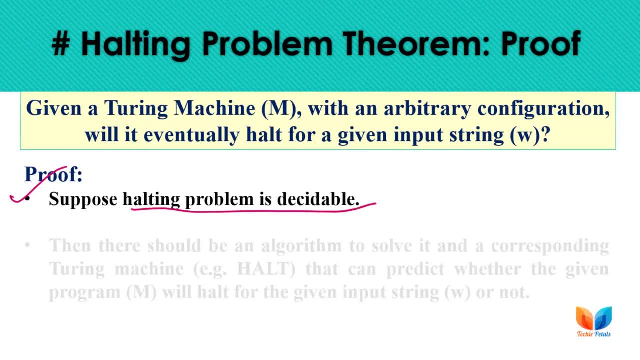 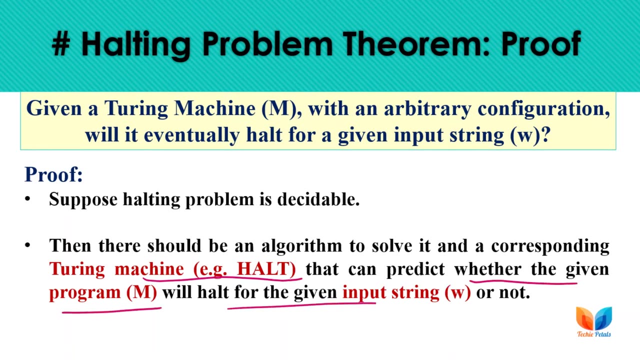 assuming that the halting problem is decidable. so we are taking the contradictory case: that halting problem is decidable and we can have such machine. we can have such machine that can predict whether the given program m will halt for the given input string or not. so we are taking the opposite case. 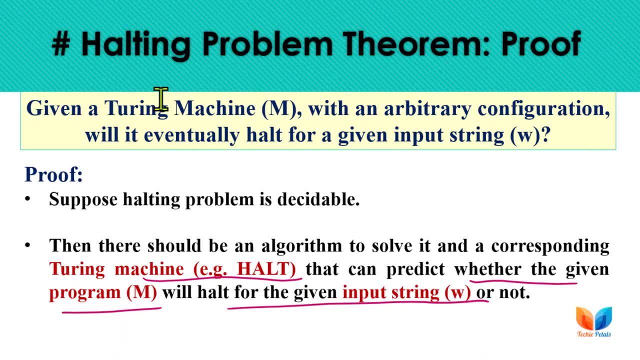 contradictory case that we can have such machine that can give the output as yes or no for the program m and w string and the input string w. so we are naming this machine as halt. we are naming such machine as halt. that we are just assuming. so here is a halt machine. 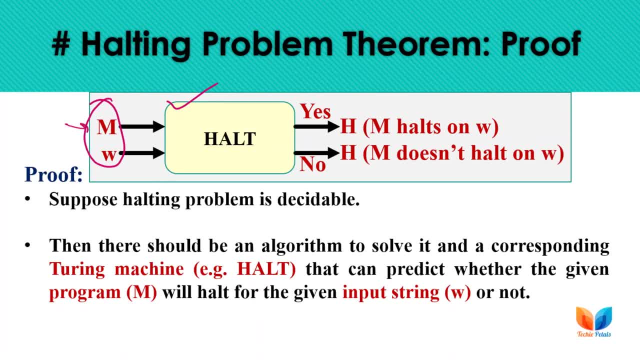 that is taking a program or a turing machine m as input and a string w as input, and it is giving the output yes if the machine m will halt for the input string and a no if the machine doesn't halt for the input string w. so this is the. 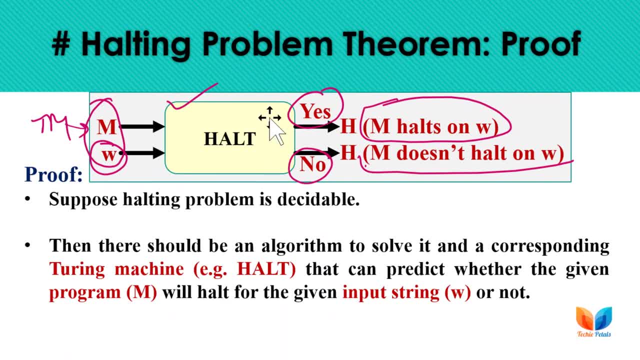 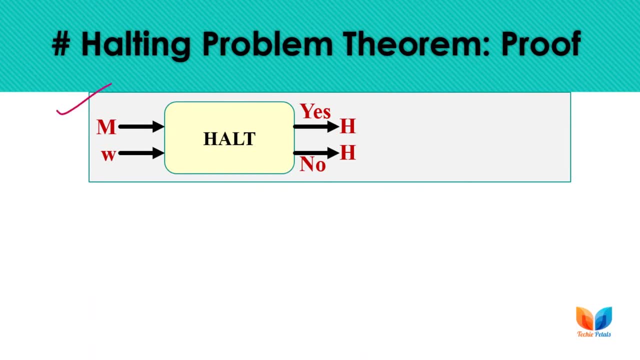 contradictory case that we are assuming such machine or a solution can exist, an algorithm can exist that can solve our halting problem. so we are just assuming that. so now this was a machine that is solving our purpose means we are assuming that such machine can exist. now this is the coding. we can say that a 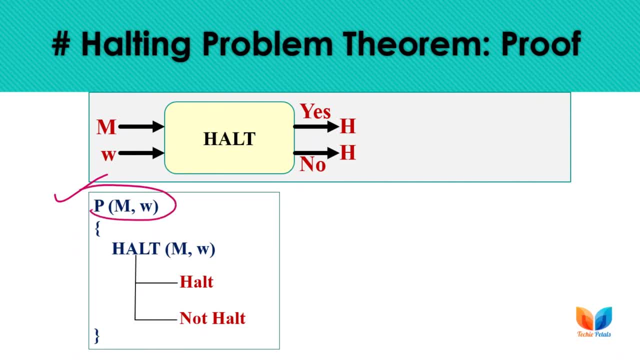 solution for this. we are having a program that is taking machine m and w as input and calling the function halt. that is our solution. means this algorithm is solving our halting problem. we are assuming this- and it will halt. it will giving a yes. so yes, for if the machine will halt and 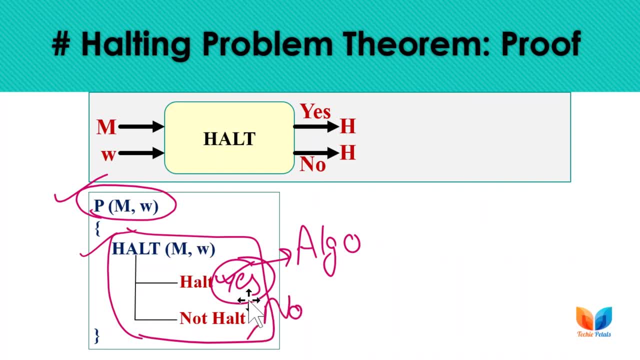 a no, if the machine will not halt for the input string w. so this problem can be solved with this algorithm: halt algorithm. we are just assuming this. now we are taking a contradictory case. so by again we are taking a contradictory case. firstly, we assume that such machine can. 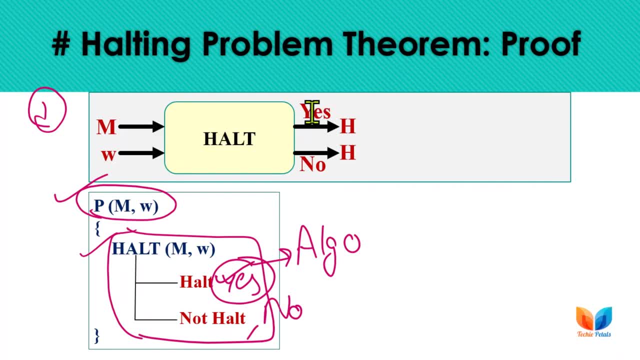 exist that can predict whether it the machine will give result or not. so first contradiction was this. next, we are taking again a contradictory machine for this machine. so as this was the machine, now we have to take a contradict for this machine, that if halt machine can exist, one halt. 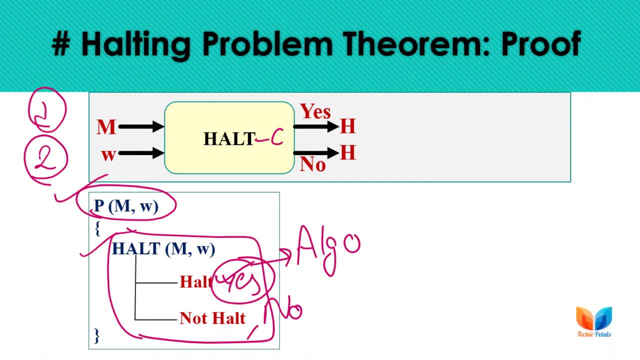 contradict, machine can also exist. by contradict we mean that here the for the yes case that machine will halt for this particular string w we are. we are assuming that we can predict that machine will halt for this particular string. but again we are adding some contradiction and new machine is named. 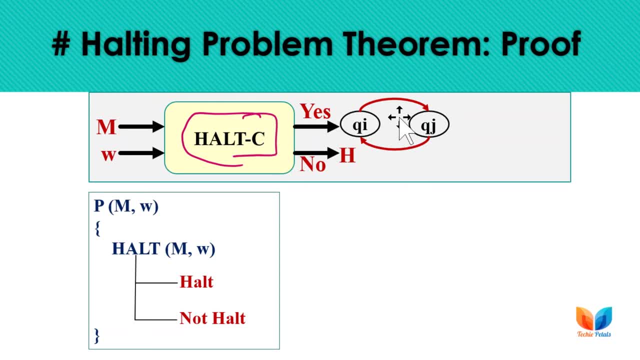 as halt contradict halt, hyphen c, and we are, we are assuming or we are contradicting the previous case by adding a infinite loop. we are adding an infinite loop here with two states as qi and qj, and these two states are moving from left to right and left, right to left. so 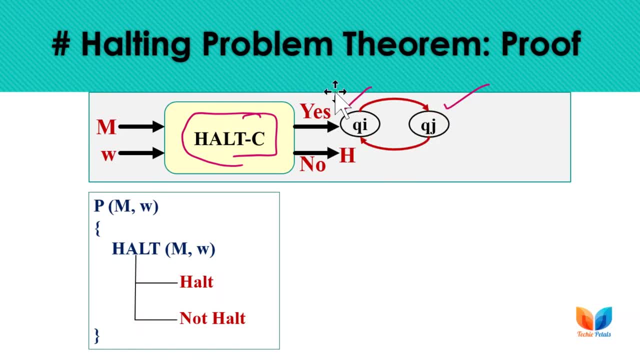 these are the transition that will loop forever. or if for the yes case means to prove yes, if we are having any of such type of loop in the machine, so for any of such type of machine, the machine will also. the machine will again comes or ending with a loop and will. 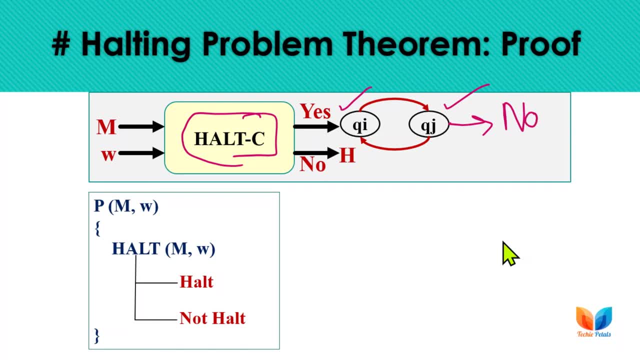 never halt will never halt. okay, so if such k, if halt machine was possible, if halt machine was possible, halt contradict machine is also possible. that for the yes case, for halt case, we again, if we are having a infinite loop, so if we are having an infinite loop for 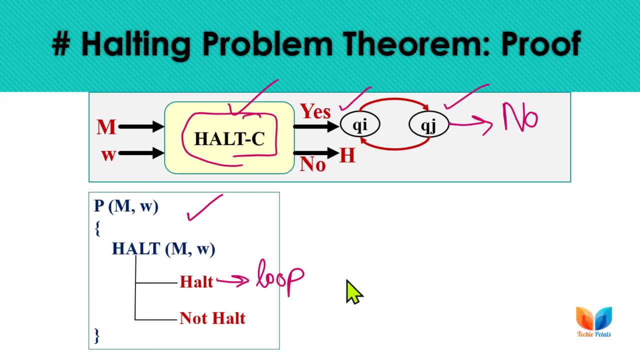 halt case as well, then the machine will also again. the machine will again enter to the uh. undecidable mode means we cannot predict whether this loop will halt or not. so this is the contradictory case here. so here is the program corresponding to this we are having. if this halter, 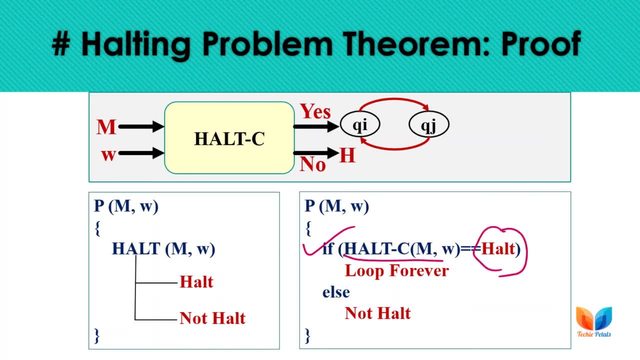 contradict machine is giving you a halt output, then it will. then it is entering into a infinite loop. by infinite loop we mean that a loop that will run forever means we can have a forever true loop while one or while two, and this loop will never end for any. 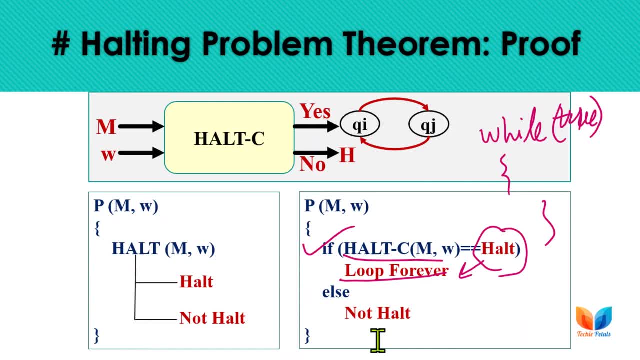 case. so and else we are having not halt means the machine will not halt, and so for contradiction, so for contradiction here, for halt case again, we are entering into the loop case. so the machine will not halt, even for the yes case. so this can also be represented in a better way than the 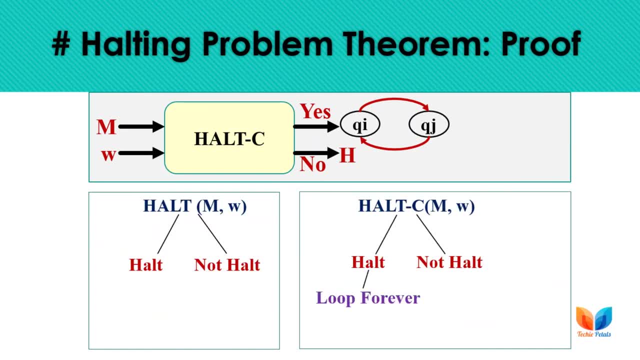 in a better way using a, using a flow diagram. like for halt we are having halt and for the hold machine we were having the two outputs as halt and not halt, and for halt contradict, we are having the same two output as halt and not halt, but for halt case we are entering to. 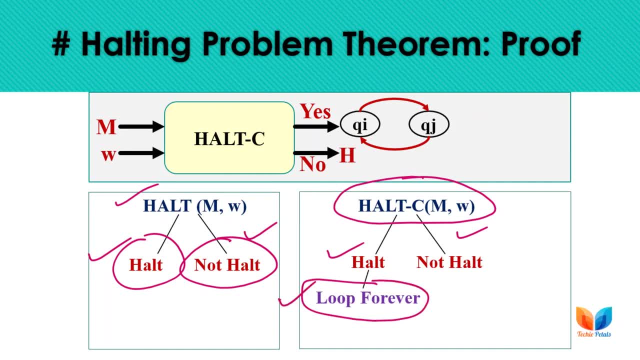 or we are adding a loop and the machine will goes to loop. uh, in goes to an infinite loop even after the halt case. so here we can say that for all other cases, for all other cases we are having, the halt state means whether we the machine will not hold. but 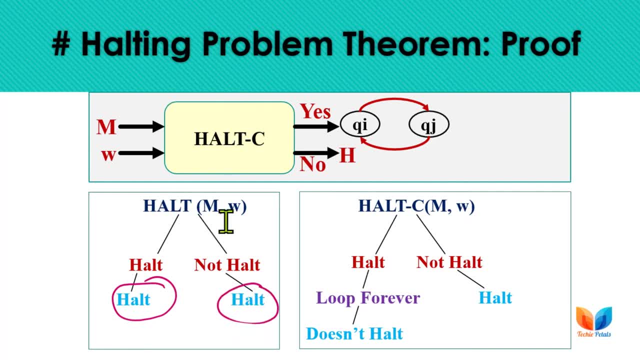 it is giving some result. so this machine, so halt. result is giving you some result means this machine is, this machine is coming to halt. state means whether this m, the, whether this m program will halt or not halt. so the we can say that ultimately this machine is in halt state okay, whether 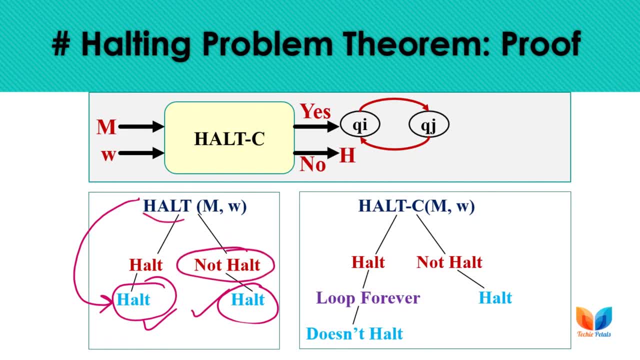 whether the m is in not halt state. but the halt machine that we have predicted or assumed to exist is halt, is halting in all the cases. but here is a hold contradict machine that is uh, for that is even for the halt case- is it is moving to the loop and it will not. 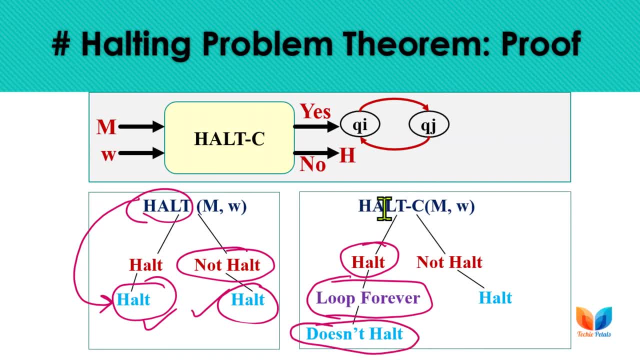 halt ever. so this machine is not going to end with any of the decision. so this machine is not going to give you any output, whether this m will halt or not. so here we have the contradiction, here we have the contradiction that the machine we assumed to give the result, the machine we 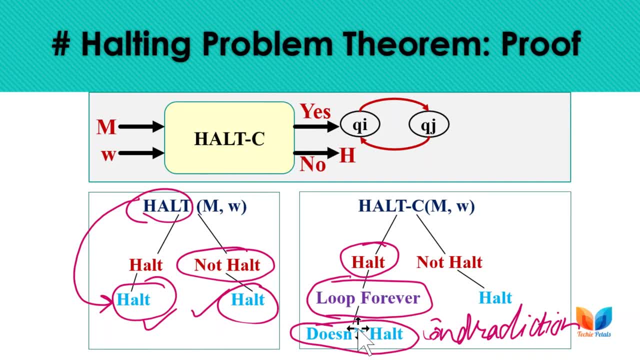 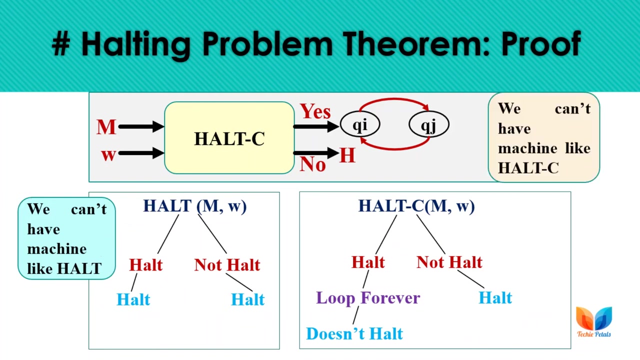 assumed to give the result, is itself going to the, going to the infinite loop, and will not give the result. so here such machine cannot exist. so we can prove by contradiction that halting problem is undecidable, as we cannot have the machine like halt and we cannot have the machine like